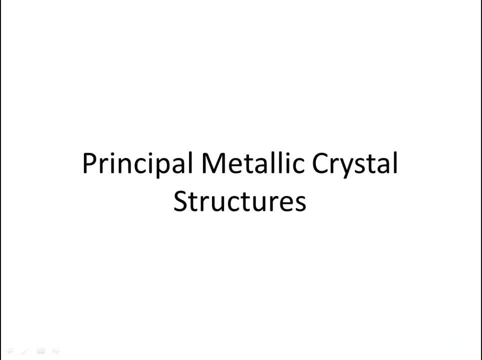 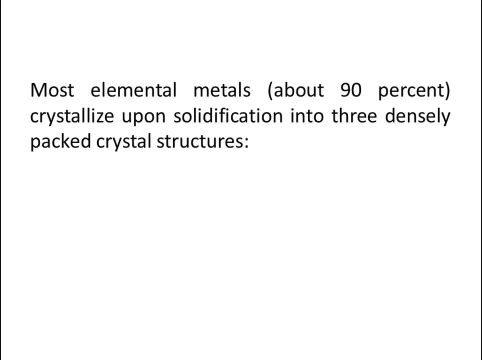 Let's talk about principal metallic crystal structures. Most elemental metals- that means around 90% elemental metals- crystallize upon solidification into three densely packed crystal structures, and the first one is body centered cubic. second one is face centered cubic and the third one is hexagonal, close packed Body centered cubic is called BCC, in short FCC centered cubic. 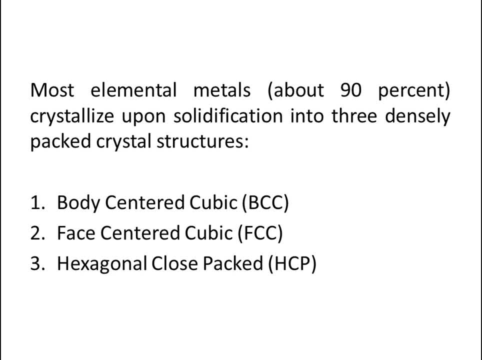 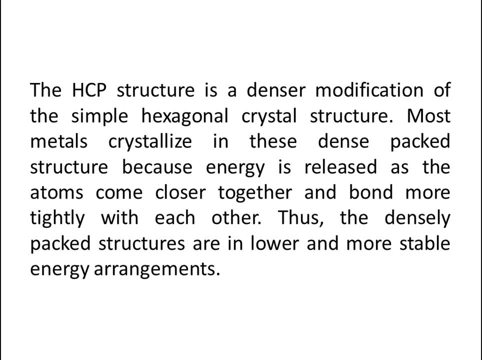 is called FCC in short, and hexagonal close packed is called HCP in short. The HCP structure is denser modification of the simple hexagonal crystal structure. Most metals crystallize in this dense packed structure because energy is not stored in the material, So the energy is stored in the 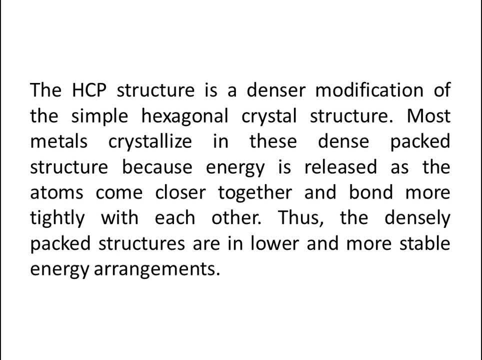 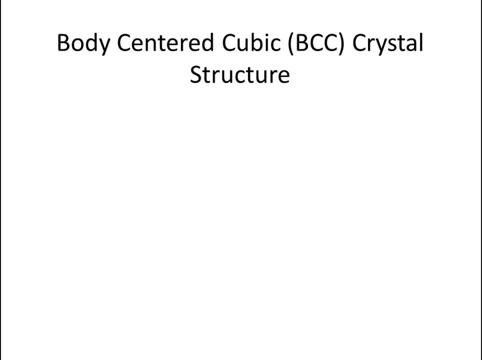 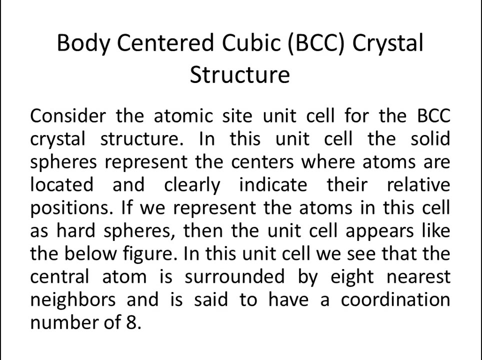 released as the atoms come closer together and bond more tightly with each other. Thus the densely packed structures are in lower and more stable energy arrangements. Let's talk about body centered cubic crystal structures. that means BCC crystal structure. Consider the atomic site unit cell for 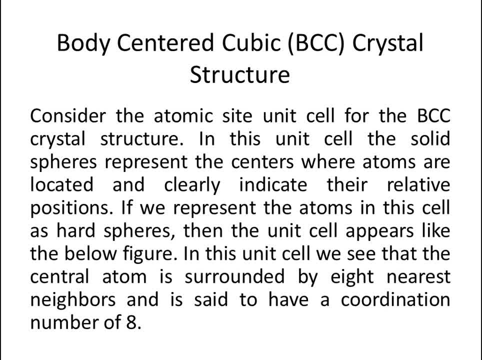 the BCC crystal structure. In this unit cell the solid spheres represent the centers where atoms are located and clearly indicate their relative positions. If we represent the atoms in this cell as heart spheres, then the unit cell appears like the bell figure. In this unit cell we see that the central 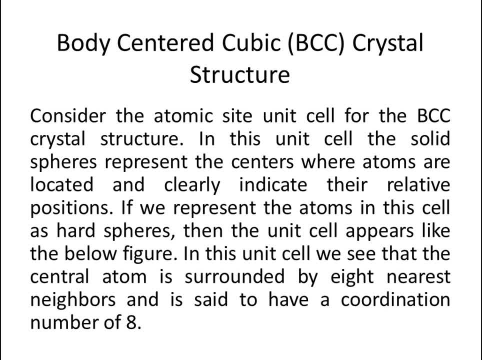 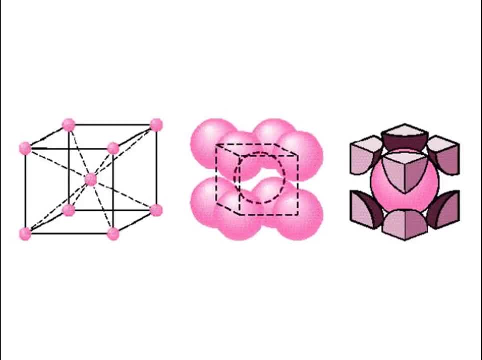 atom is surrounded by eight nearest neighbors and is said to have a coordination number of eight. Now check the figure. So in case of body centered cube, the atom is at the body and there are eight atoms at the corner and if we check this one, so this is a simple cubic and this is the cubic. 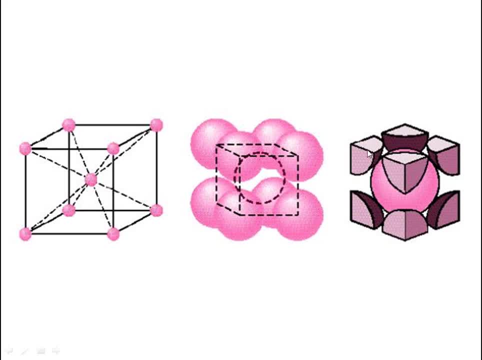 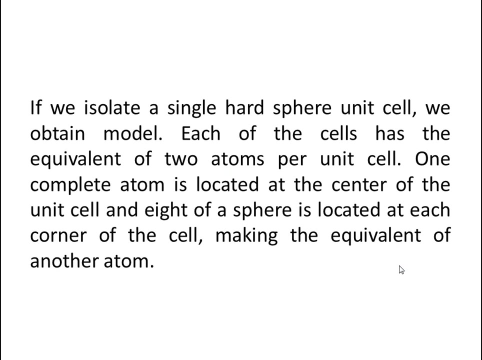 structure actually. So at the center there is one atom and these are the one eighth part of the atom. so this, there is one atom and these eight make another atom. so there are two atoms in this BCC structure If we isolate a single heart. 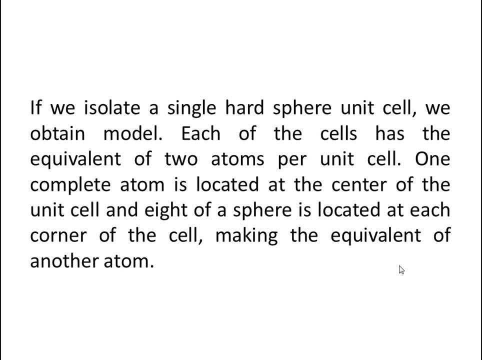 sphere unit cell, we obtain model. Each of the cells has the equivalent of two atoms per unit cell. One complete atom is located at the center of the unit cell and eight of a sphere is located at each corner of the cell, Making the equivalent of another atom. Let's talk about face centered cubic crystal. 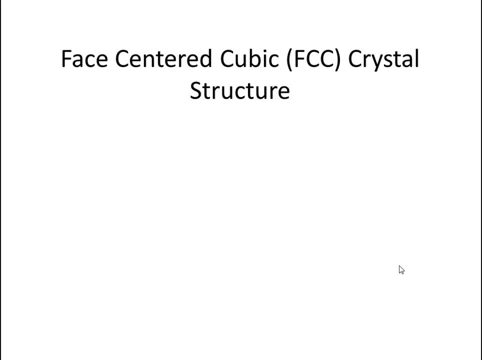 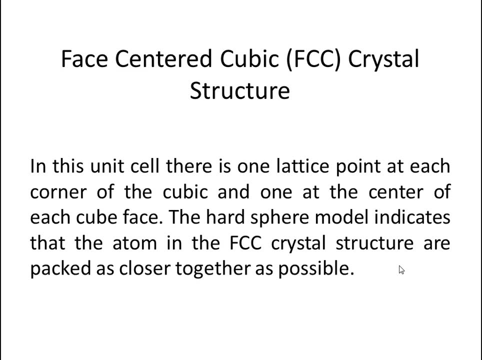 structure. that means FCC crystal structure. In this unit cell there is one lattice point at each corner of the cubic and one at the center of each cube face. The heart sphere model indicates that the atom in the FCC crystal structure are packed as closer to the other end and the two other end are claused, So it is applicable that each one is. 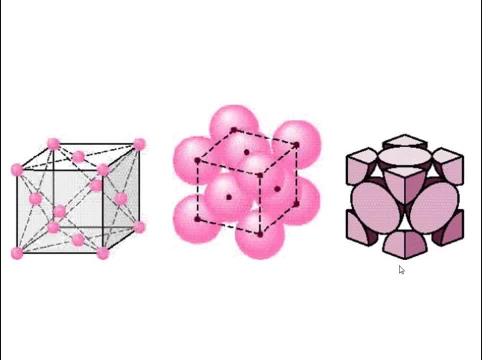 end of the unit cell and one end of the cube. If the dues are closed, then the unit cell is not as possible. and this is the structure. so, uh, these atoms are at the face and these atoms are at the corner. and if we check the arrangement that this is the arrangement f, and if we isolate the just, 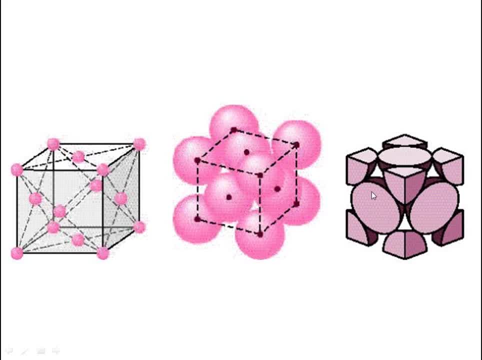 one cube. so this is the cube, so these are the face. so this one and the opposite one makes one atom. this one and the opposite one make another atom. this one and opposite one make another atom. so they are here, we get six atoms. and this one, eighth position, make another atom. so there are four atoms. 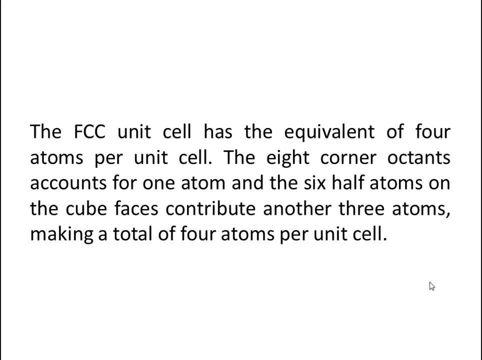 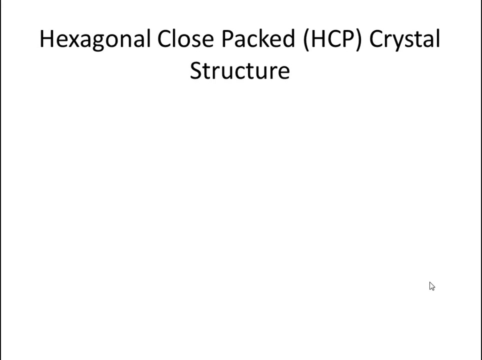 in fcc structure cube. the fcc unit cell has the equivalent of four atoms per unit cell. the eight corner octants account for one atom and the six half atoms on the q faces contribute another three atoms, making a total of four atoms per unit cell. let's talk about hexagonal close pack crystal structure. that means acp crystal structure, the. 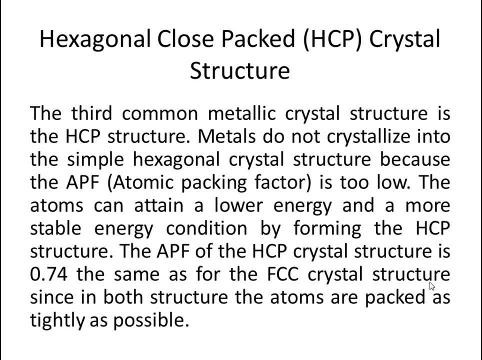 third common metallic crystal structure is the acp structure. metals do not crystallize into the simple hexagonal crystal structure because the apf, that means atomic packing factor, is too low. the atoms can attain a lower energy and a more stable energy condition by forming the hcp structure, the apf of the hcp.